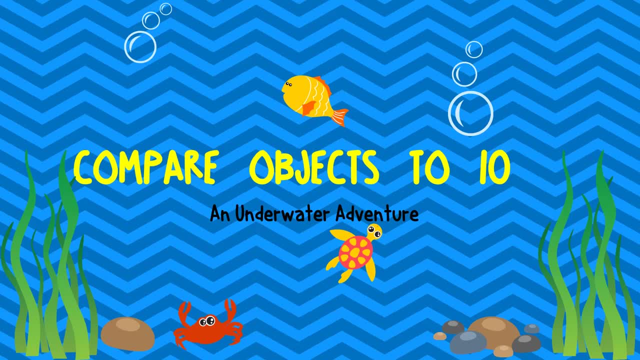 Hello and welcome back. Today I have a lesson on comparing objects to 10.. Now, this is a beginner's lesson, so we are not going to have any numbers. There's going to be no numerals or digits, whatever you want to call them. We are only going to talk about objects, a group of objects that we 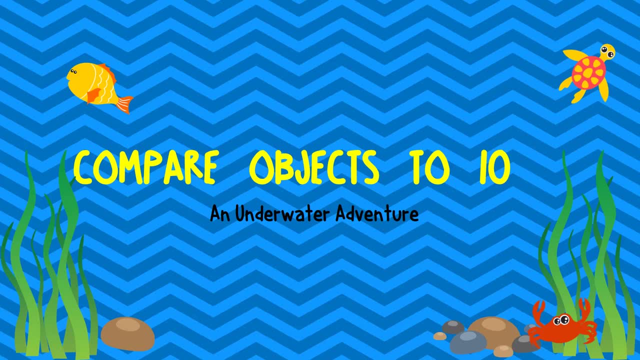 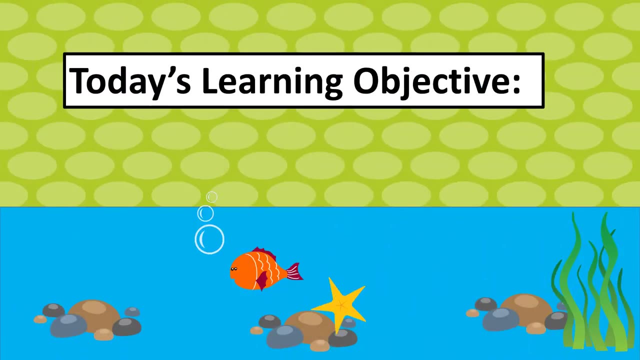 will be comparing, So if this is the video that you're looking for, then keep watching Today's learning objective. Now, this is what we're going to be able to do by the end of the lesson today. I always have my students repeat after me. 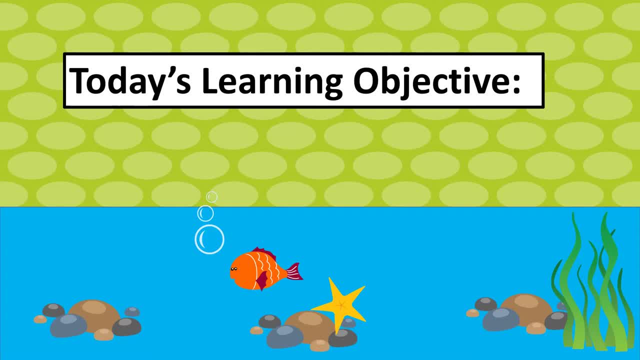 so that they are aware of what they are going to learn. I can compare groups of objects By using the words greater or least. Now you're probably wondering what the words greater or least mean, and we're going to talk about that next. 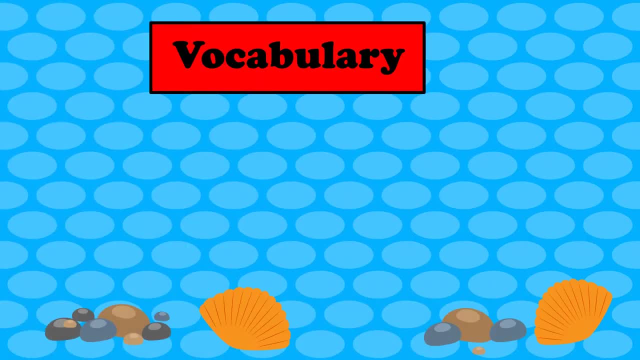 Vocabulary. Vocabulary is so important when you begin a new concept, So we're going to go over these words. Greater, Everybody say greater. Now there are some other words that are very similar to the words greater and they are more, You could say there. 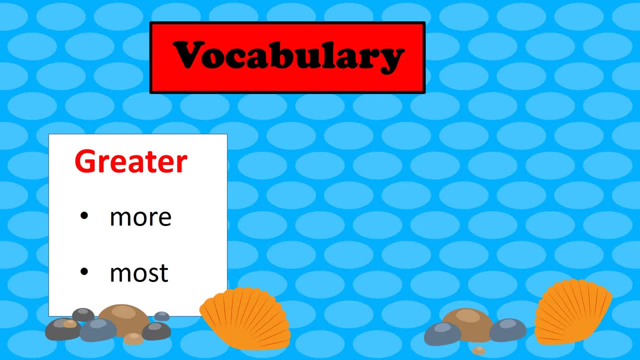 are more, and you also could say most, Which one has the most. But in today's lesson we are going to use the academic language greater, and we're also going to use this word least. Everybody say least, Great, And there are some other words that are very similar to the word you said. 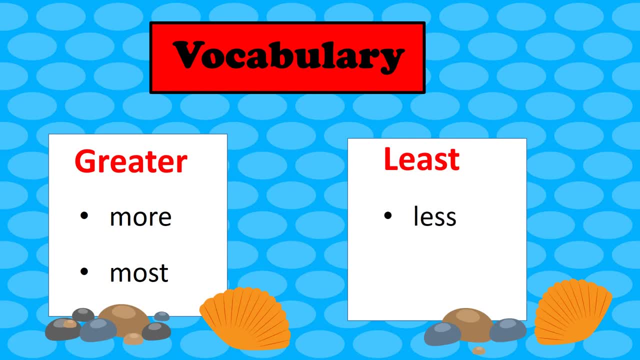 Say, and you were. But, like I said earlier, the words that we are going to use in our lesson today greater and least. Now, before we start, there are some kind of learning mistakes. Now, before we start, there are some kind of learning mistakes. 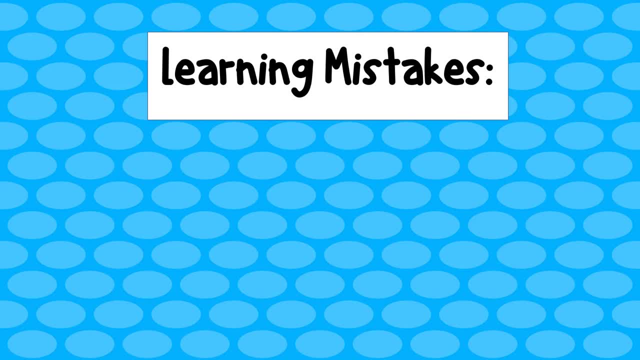 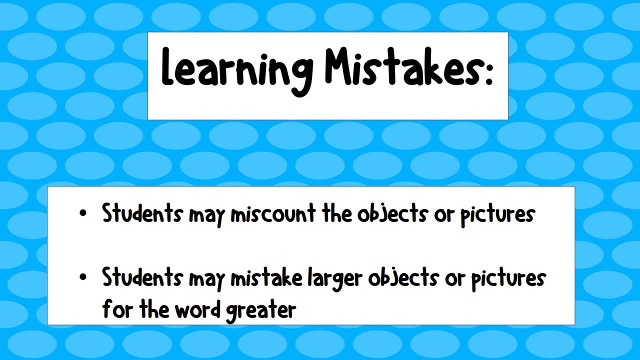 that students make. These are the most common. The first one is that students may miscount the objects or the pictures. Now, if they don't have one-to-one correspondence, then they probably need to start with counting and one-to-one first, before they start comparing, because then they might miscount and 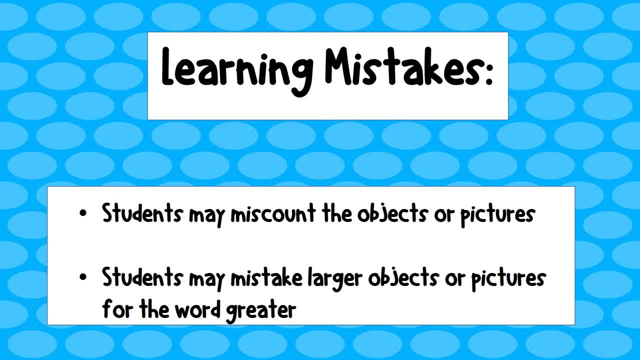 come up with the wrong number and then they're not going to be able to compare. Another one is that students may mistake larger objects or pictures for the word greater. Now, just because the object is larger doesn't mean that it is greater. So we're not talking about size of the objects, we're talking about the 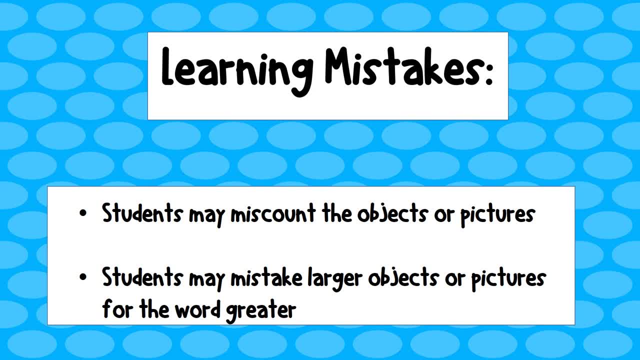 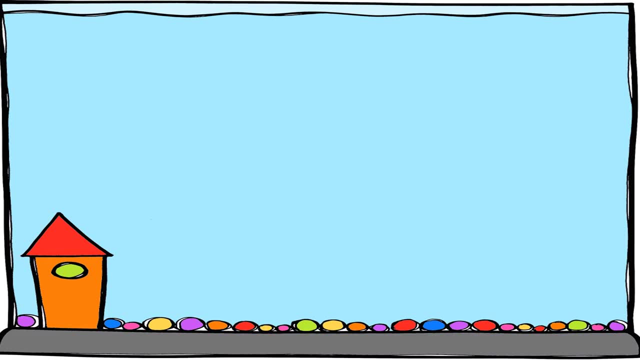 quantity, So make sure that your students know the difference between larger and greater. Ok, let's go ahead and start. So here is my learning mat and we're going to see what animals we come across. Let's start here with number one: turtle. We have one turtle. 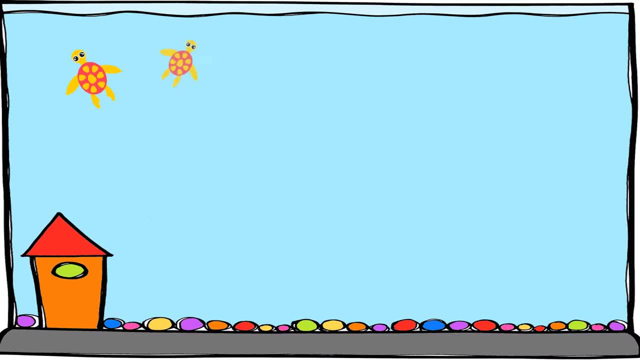 Let's go ahead and count with me one, two, three, four, five, four, five, four, five, six. we have six turtles, and then there's one seahorse and two seahorses. I want to know which one is greater. let's think about this. well, we know there are six. 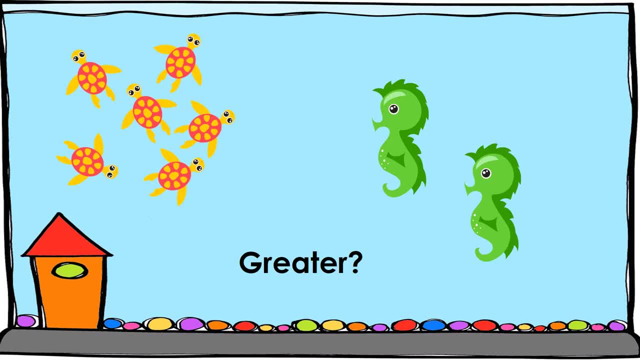 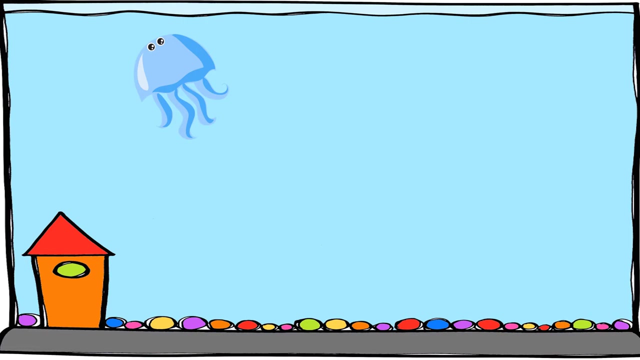 turtles and there is two seahorses. what do you think which one is greater? right, it's the turtle, because there are six, and six is greater than two another one: there's one jellyfish, two jelly fish, three, four, five, five jellyfish. and then there's 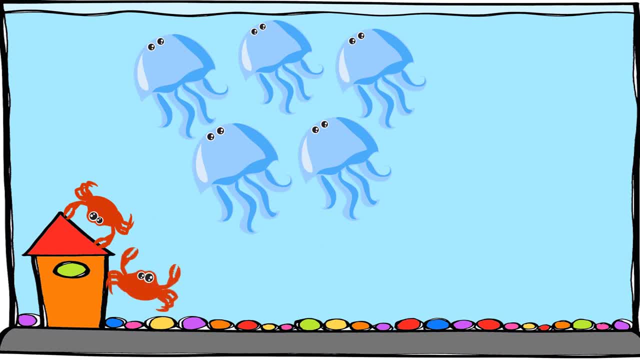 one crab, two, three, four, five, six, seven, Seven crabs. I want to know which one has the least. Hmm, let's think about this: Five jellyfish and seven crabs. What do you think? Which one has the least? 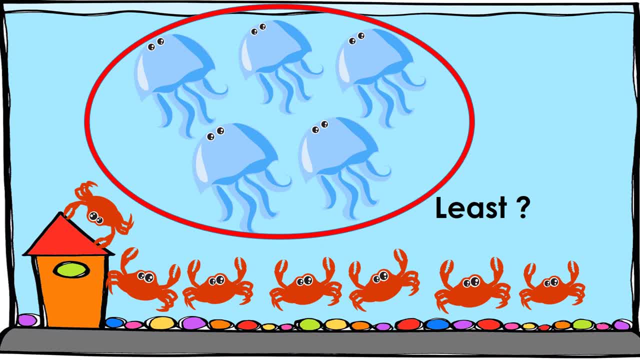 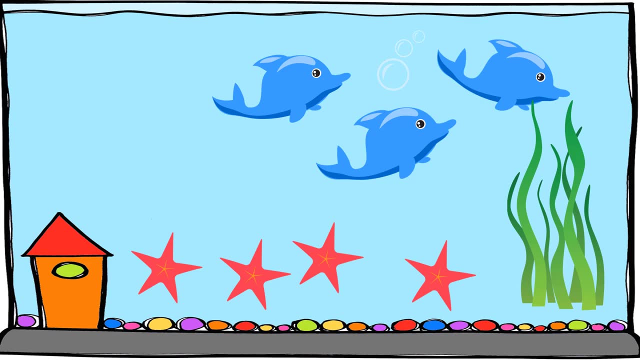 You're right, The jellyfish are the least, because five is less than seven. Let's try another one This time. you already see the pictures. There are some dolphins and there are some starfish. Hmm, I want to know which one is greater. 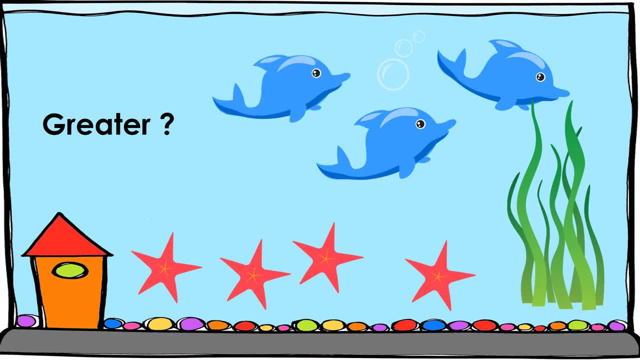 Let's count One dolphin, Two dolphins, Three dolphins. Let's count the starfish: One, two, three, four. Which one is greater? You're right. The jelly fish are the least. You're right, They're greater. I know they're. 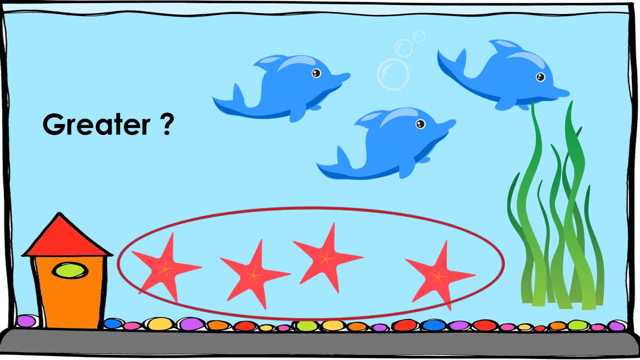 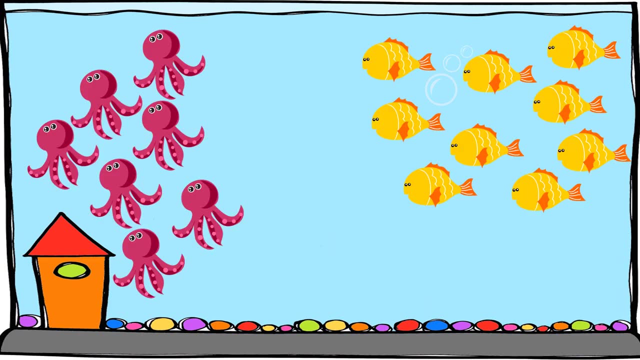 right, it is the starfish. there are four starfish and only three dolphins. you're doing really good. let's try another one this time. we have some octopus and we have some fish. let's see how many. there are one, two, three, four, five, six, seven, seven octopus and let's see how many fish.